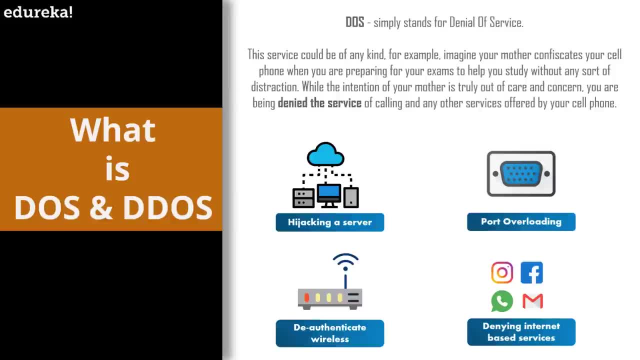 While single machine attacks are much easier to execute and monitor, they are also easy to detect and mitigate. To solve this issue, the attack could be executed from multiple devices spread across a specified area. Not only does this make it difficult to stop the attack, but it also becomes 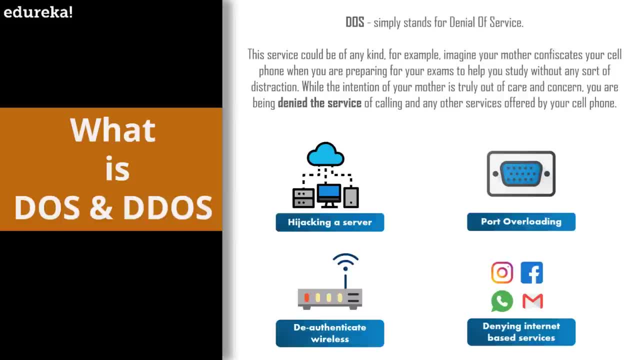 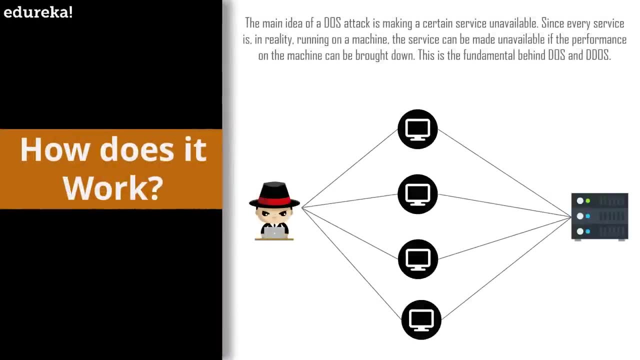 near impossible to point out the main culprit. Such attacks are called distributed denial of service or DDoS attacks. Now let's see how they work. The main idea of a DDoS attack, as explained, is making a certain service unavailable, Since everything that is attacked is in reality running. 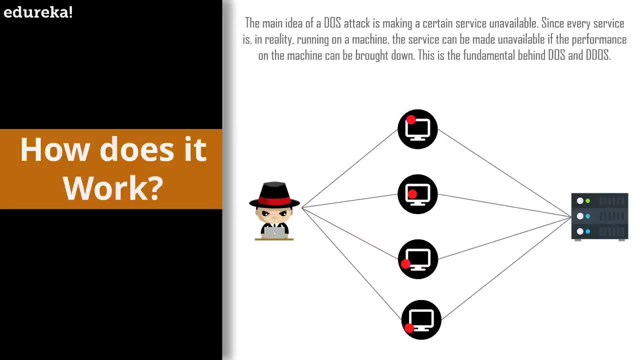 on a machine. the service can be made unavailable if the performance of the machine can be brought down. This is the fundamental behind DOS and DDoS attacks. Now some DOS attacks are executed by flooding servers with connection requests until the server is overloaded and is deemed useless. Others are executed by sending unfragmented packets to a 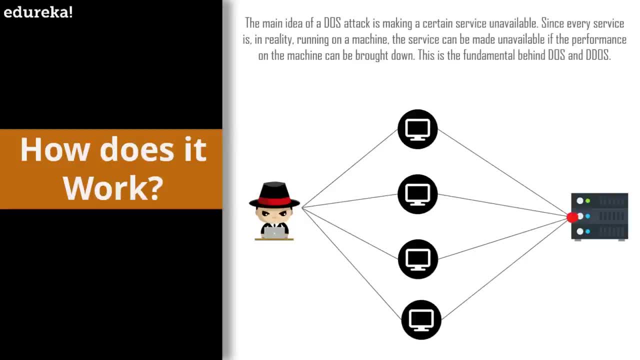 server which they are unable to handle. These methods, when executed by a botnet, exponentially increase the amount of damage that they are doing and their difficulty to mitigate increases in leaps and bounds. To understand more about how these attacks work, let us look at the different. 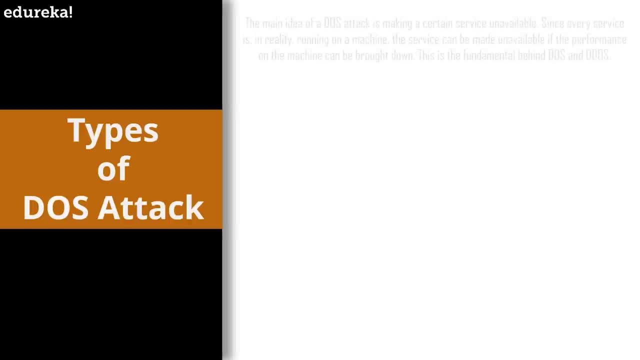 types of attacks. Now, while there are plenty of ways to perform a DDoS attack, I'll be listing down the more famous ones. These methodologies have become famous due to their success rate and the damage they have caused over time. It is important to note that, with the 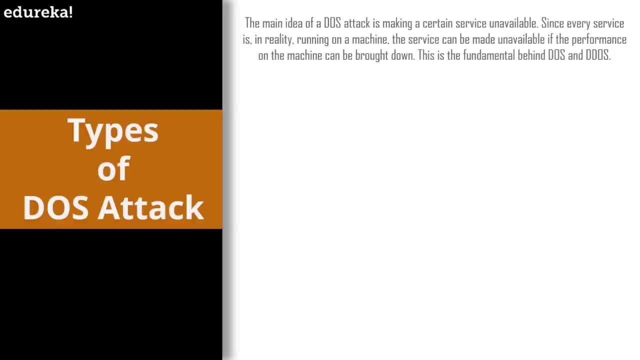 advancement in technology, the more creative minds have devised more devious ways to perform DDoS attacks. Now the first type of methodology that we're going to discuss is called ping of death. Now, according to the TCP IP protocol, the maximum size of a packet can be 65,535 bytes. The ping. 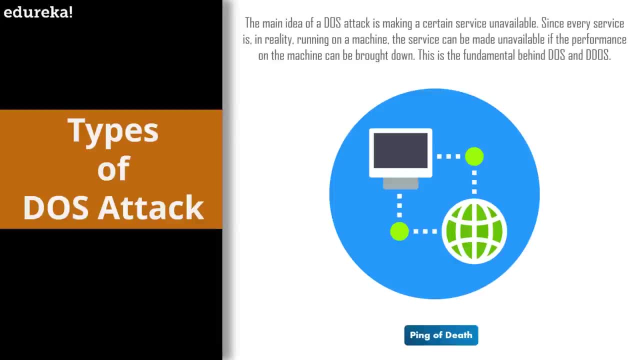 of death attack exploits this particular fact. In this type of attack, the attack is performed by sending packets that are more than the max packet size. when the packet fragments are added up, Computers generally do not know what to do with such packets and end up freezing, or sometimes 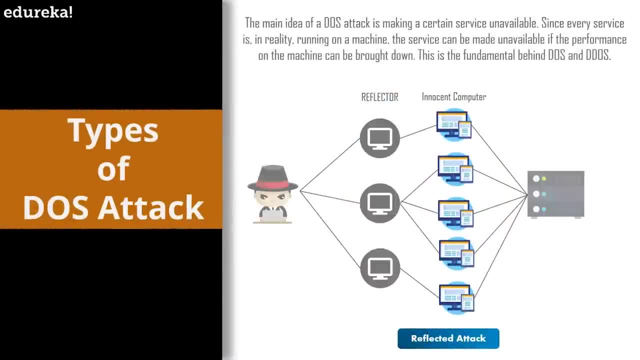 crashing entirely. Then we come to reflected attacks. This particular attack is, more often than not, used with the help of a botnet. The attacker sends a host of innocent computers a connection request using a botnet, which are also called reflectors. Now, this connection that comes. 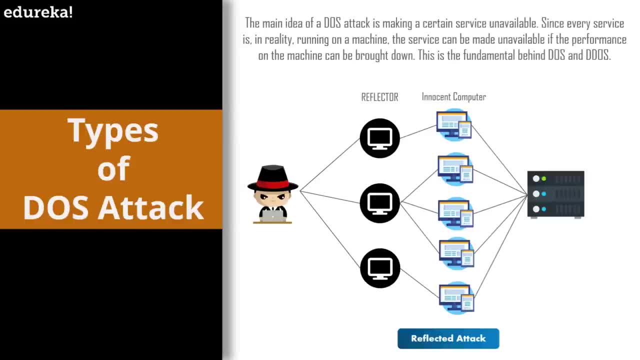 from the botnet looks like it comes from the victim, and this is done by spoofing the source in the packet header. This makes the host of computers send an acknowledgement to the victim computer, Since there are multiple such requests from the different computers to the same machine. 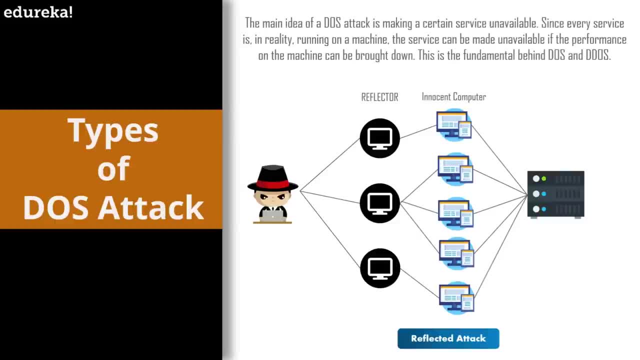 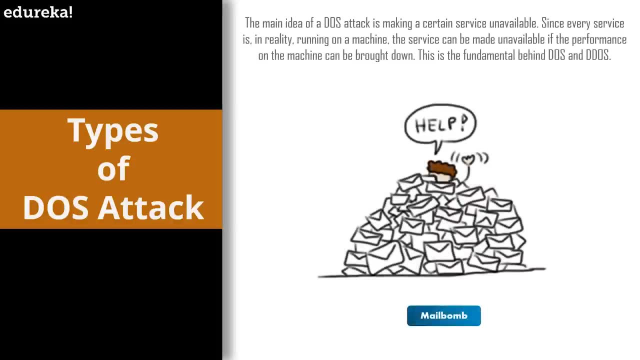 this overloads the computer and crashes it. This type of attack is also known as a smurf attack. Another type of attack is called mail bomb. Now, mail bomb attacks generally attack email servers. In this type of attack, instead of packets, oversized emails filled with random garbage values are sent. 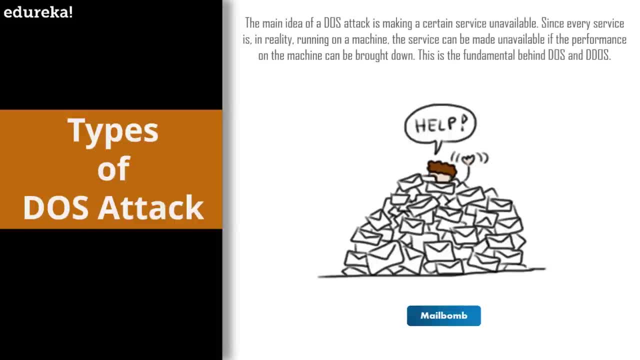 to the target's email server. This generally crashes the email server due to a sudden spike in load and the attack is called mail bomb. Now, mail bomb attacks generally attack email servers. This generally crashes the email server due to a sudden spike in load and the attack is called mail bomb. 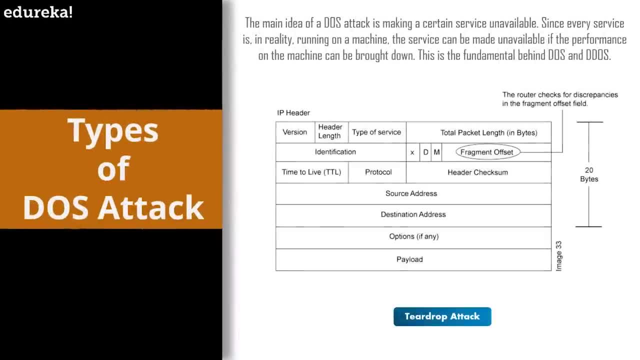 And renders them useless until fixed. Last but not least, we have the teardrop attack. So in this type of attack, the fragmentation offset field of a packet is abused. one of the fields in an IP header is the fragment offset field indicating the starting position or offset. 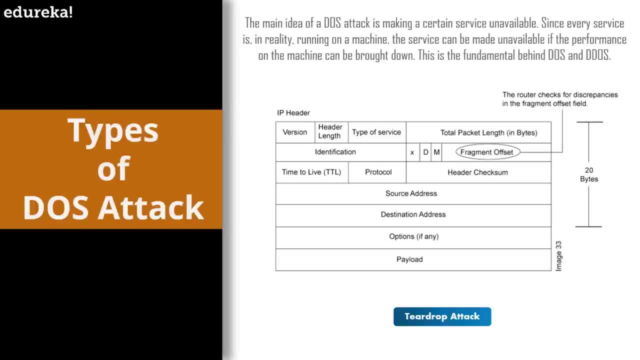 of the data contained in a fragmented packet relative to the data in the original packet. if the sum of the offset and the size of one fragmented packet differs from that of the next fragmented packet, the packets overlap. Now, when this happens, the server, vulnerable to teardrop attacks, is unable. 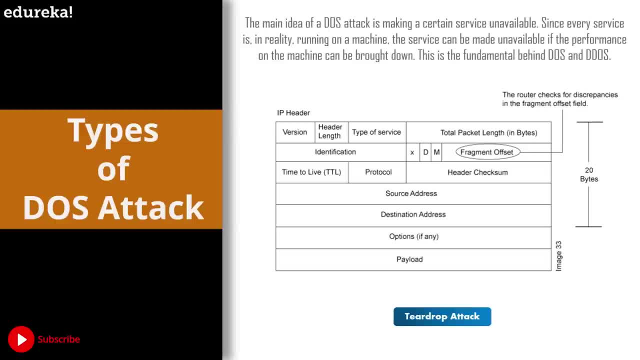 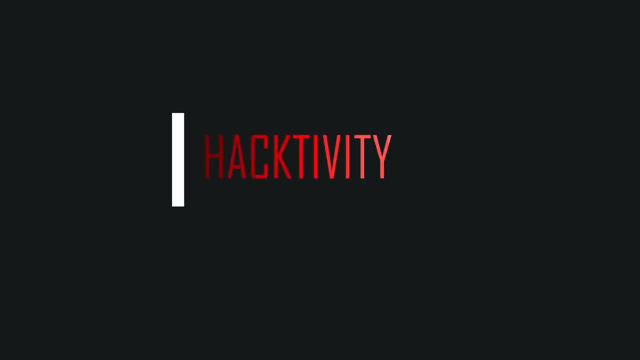 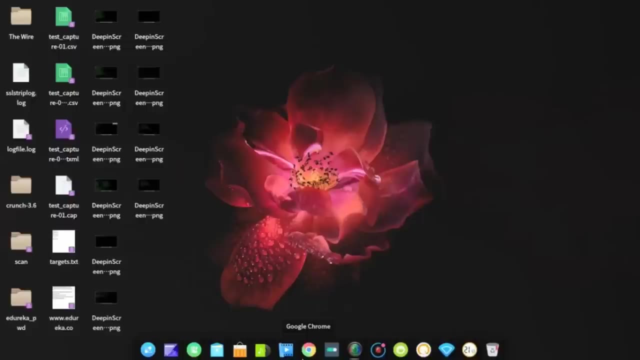 to reassemble the packets, resulting in a denial of service condition. okay, so that was all the theoretical portion of this video. now it's time to actually perform our very own DDoS attack. okay, so now that we finished the theoretical part of how DDoS actually works and what it actually is. 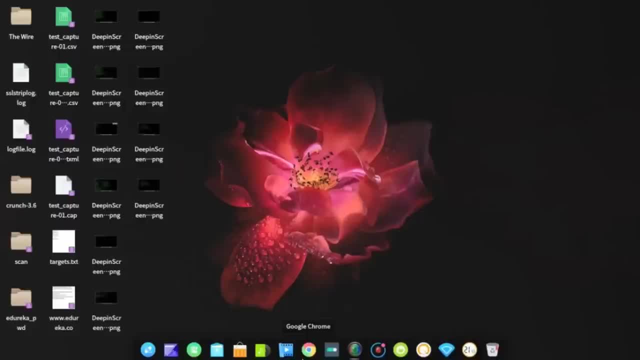 with its different types. let me just give you guys a quick demonstration on how you could apply a denial of service attack on a wireless network anywhere around you, like this could be somewhere like Starbucks where you're sitting, or this could be a library also, or your college institution. 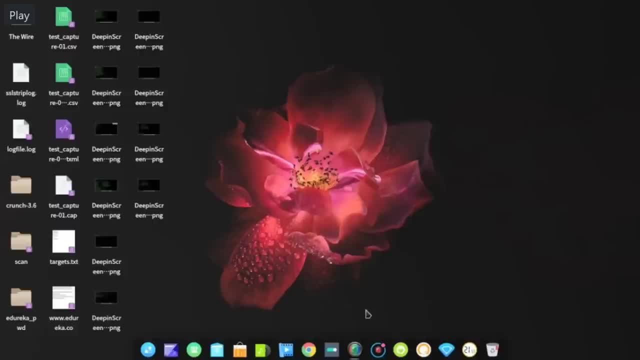 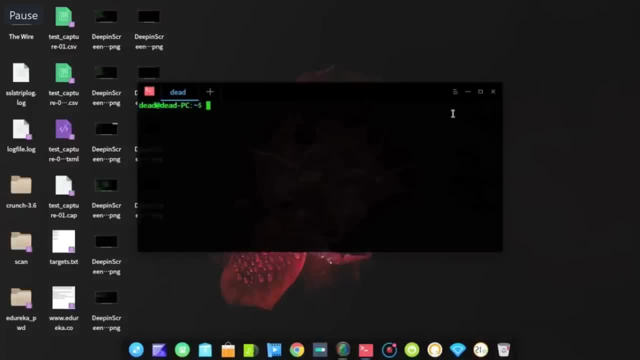 no matter where you're sitting, this procedure will work. so the first thing we want to do is actually open up a terminal, as because we will be doing most of our work on a command line basis. now, for this particular demonstration, we will be actually using two tools. first is AircrackNG. 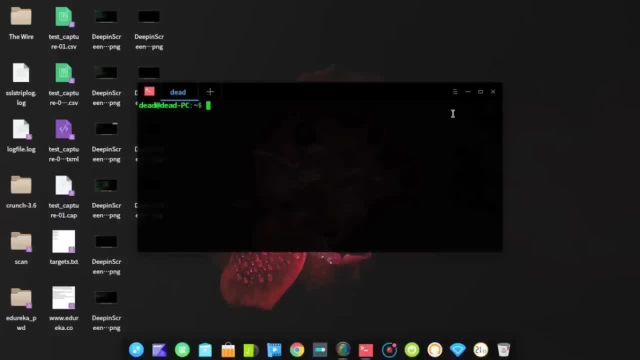 which is a suite of tools which contains AircrackNG, AirMonNG, AirReplayNG and AerodumpNG. so these are the four tools that come along with it, and the second one that we'll be using is called MapChanger. okay, 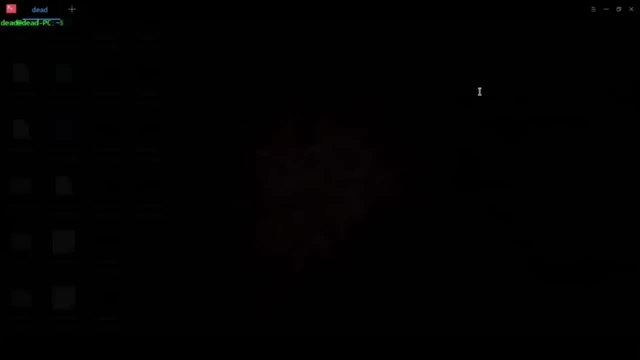 so let me just put my terminal on maximum so you guys can see what I'm actually writing out. so first thing we want to do is actually log in as a root, so let me just do that quickly. so we need to log in as root because most of the stuff that we're going to do right now will need administrator. 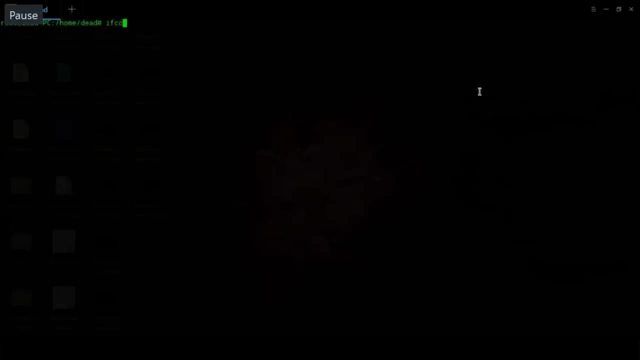 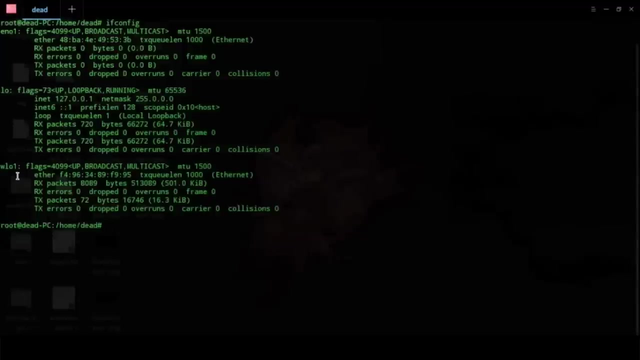 access. now the first thing we want to do is check out our wireless network cards name, and we can do that easily by typing ipconfig. now you can see that my wireless card is called WL01 and we get the MAC address and we also get the ipv6 address. so that's my wireless network card and we'll be actually. 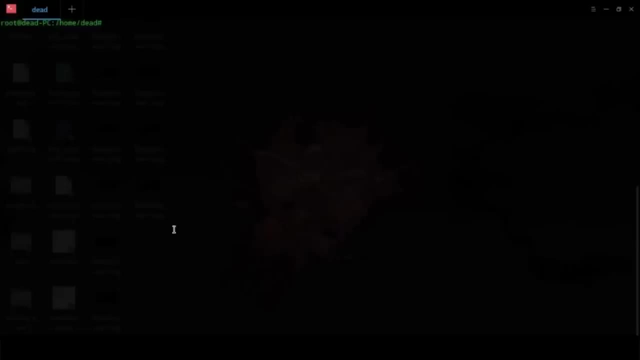 setting that up in Monitor mode. now, before we actually go into and startup our network card in Monitor mode, let me just show you how you can install the two tools that I just spoke about, that is, AircrackNG and MacChanger. so to install AircrackNG, you can just go. 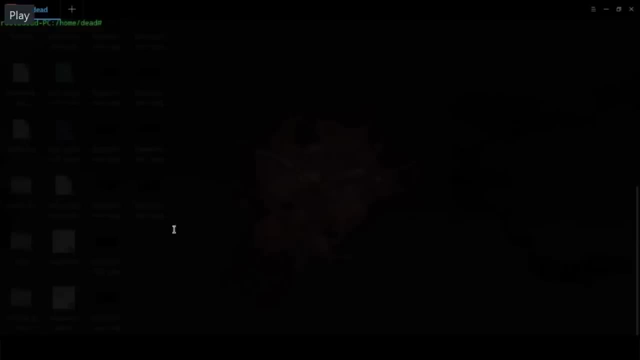 app and network card open. fliesateerme jumped and six times just made a then to connect it to aircrack and get back back to where it' apt-get install aircrackng, hit enter And this should do it for you. 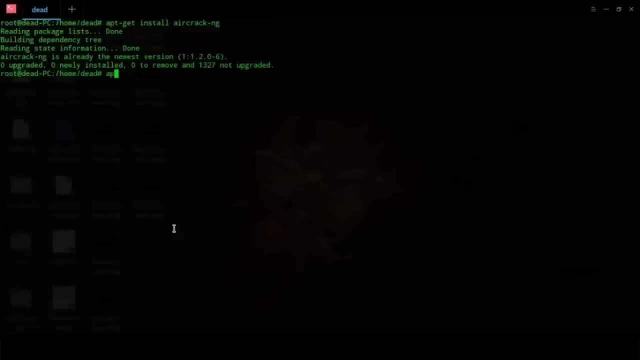 I already have it installed, so it's not gonna do much To install Mac Changer. you could just go the same command, that is, apt-get, install macchanger, And you can check if both the tools have been installed properly by opening the manual pages. 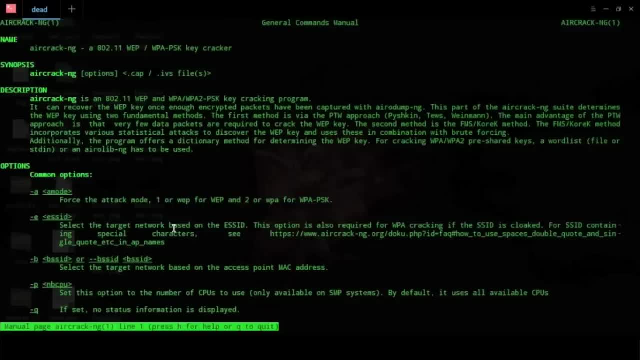 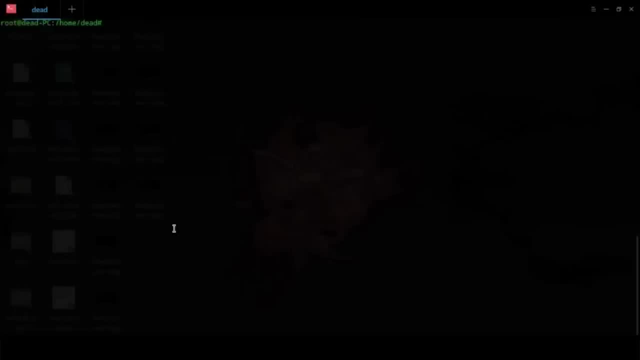 by typing man aircrackng, And this will open up the manual page for you. And let's also do the same for Mac Changer. So what we're gonna do first is set up our network interface card into monitor mode. So to do that, all we have to do is type ifconfig. 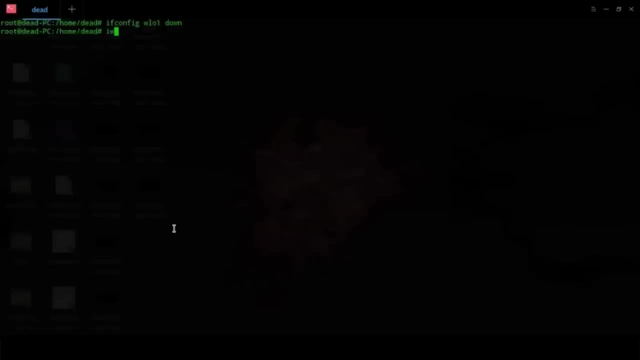 And we need to put our network interface card down. So we go wl1 down And with the command iwconfig we go mode monitor. Don't forget to specify the interface that you're working on. So iwconfig wl1 mode monitor. 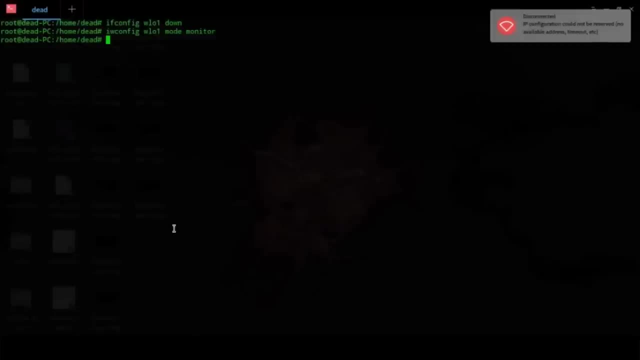 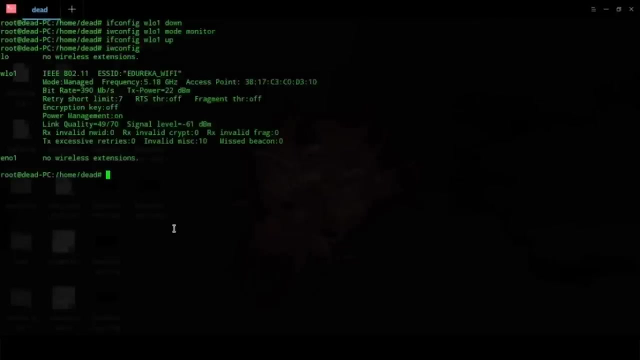 And all you have to do now is put it back up. So what we are gonna type is: ifconfig wl1 up. You can check the mode. It'll say managed if it's in monitoring mode. So, as you guys can see, it says mode managed. 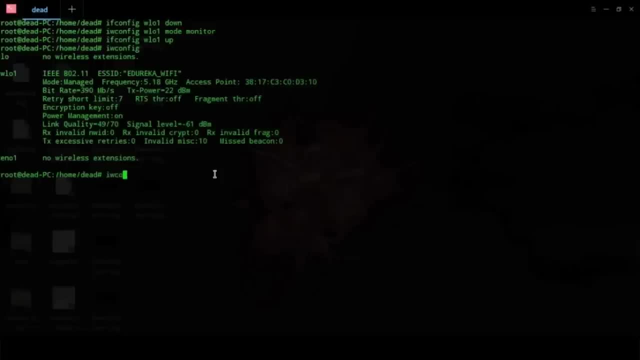 So that's how we're gonna go ahead. So you can check that just for your own purposes. So we can also check for only wl1 by specifying the interface, Or you could also check the mode only by passing it through a pipe function. 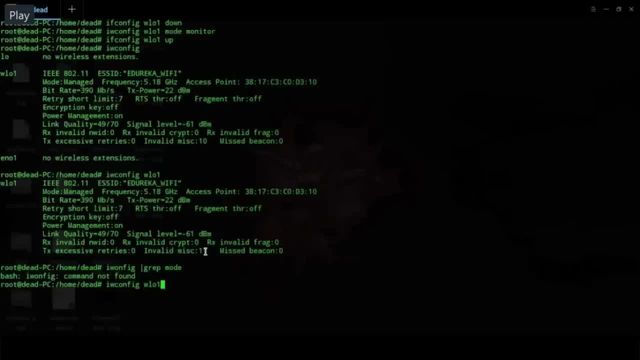 and that is using grep mode. So iwconfig wl1, grep and mode. Well, mode begins with a capital M, so that's how you would probably return it. So, as you guys can see, that has returned the mode for us. I've gone along with the access point and the frequency. 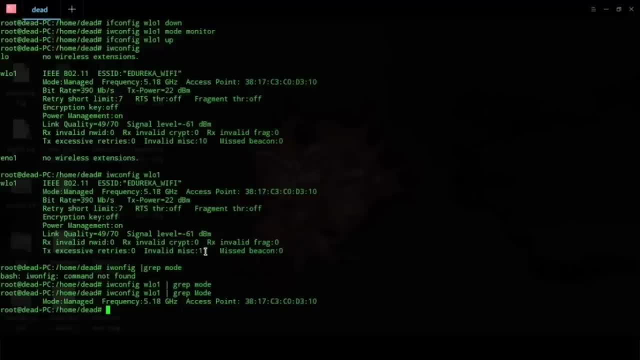 Okay, so that was a little fun trivia on how you could fetch the mode from a certain command that like iwconfig, by passing it through a pipe and grepping it with mode. Grep basically means grab. Okay, so now moving on. we'll get to the more important stuff now. 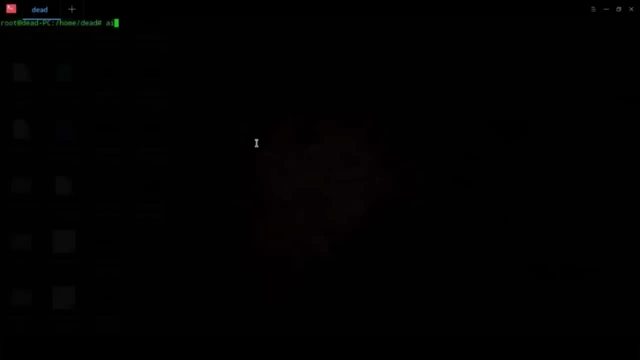 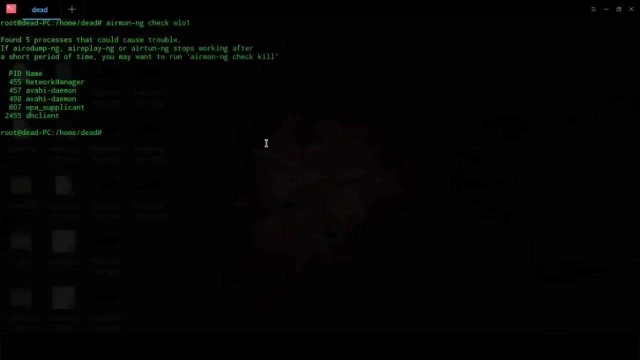 So, firstly, we need to check for some sub-processes that might still be running and that might actually interfere with our scanning process. So to do that, what we do is airmonng check and then the name of the interface. Now, as you guys can see, 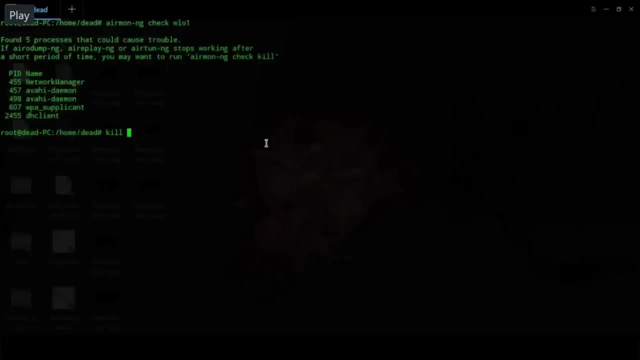 I have the network manager that is running out here and we need to kill that first, and that can be easily done by going kill with the PID. After that you can run a general command called airmonng, check and kill. So whatever it finds it will kill it accordingly. 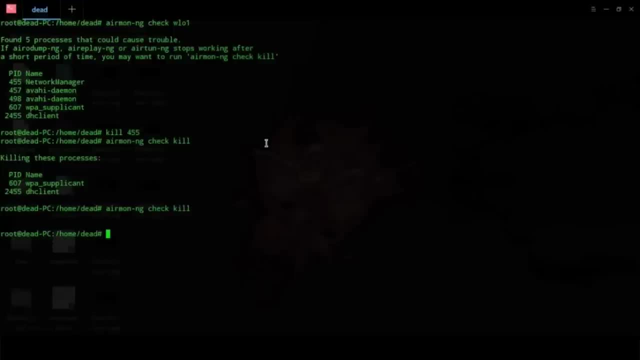 and when it produces no results like this, that means you're ready to go, as there are no sub-processes running that might actually interfere with our scan. Now what we want to do is we want to run a dump scan on the network interface card. 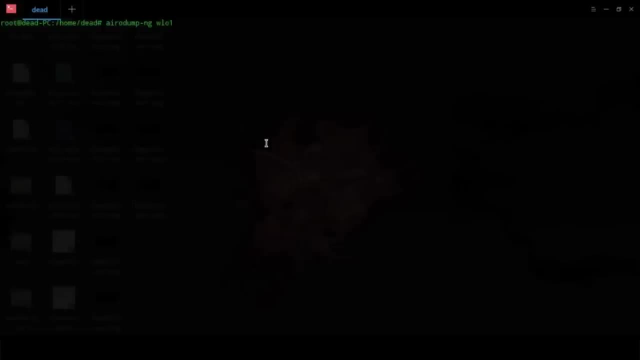 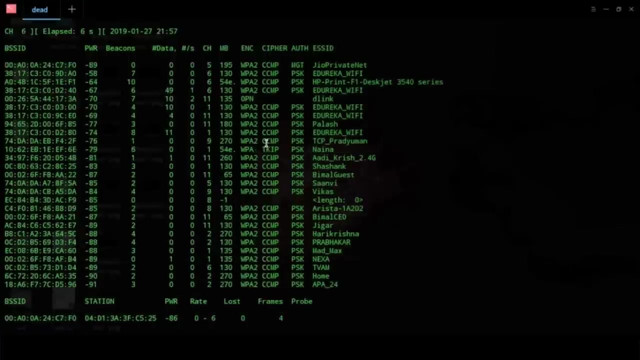 and check out all the possible access points that are available to us. So, as you guys can see, this produces a bunch of access points and they come with their BSS IDs. They also have the power, which is the PWR, That is, the power of the signal. 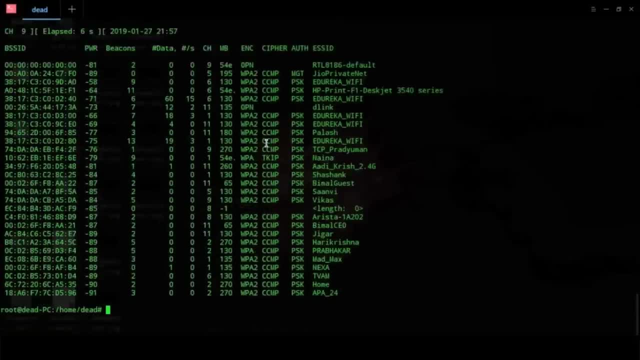 and let me go down back again. So yeah, you can see the beacons, You can see the data, You can see the channels available and what the BSS ID is. it's the MAC, the MAC ID that is actually tied in with the ESS ID. 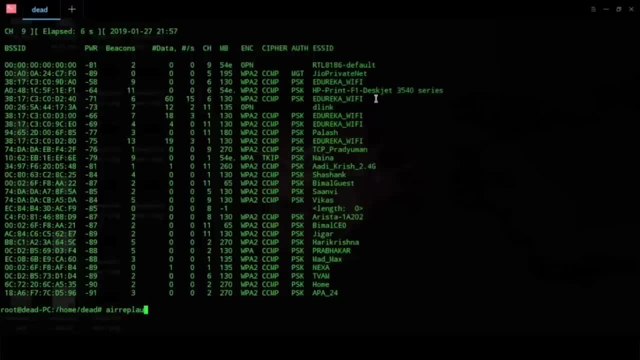 which basically represents the name of the router. Now what we want to do from here is we want to choose which router we want to actually DOS. Now the whole process of DOSing is actually: we will continuously deauthenticate all the devices that are connected to it. 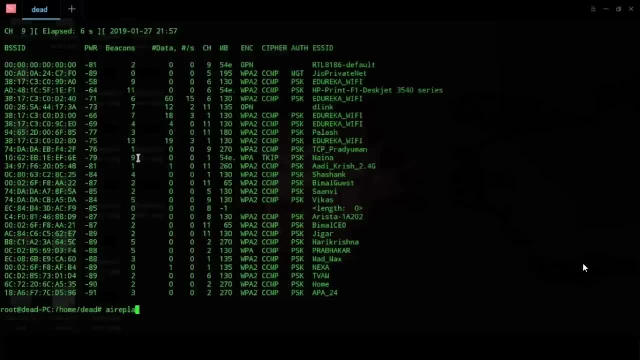 So for now I have chosen Edureka Wi-Fi to actually DOS out, and once I send a deauthentication broadcast, it will actually deauthenticate all the devices that are connected to it. Now this deauthentication broadcast is done with a tool called Air Replay. 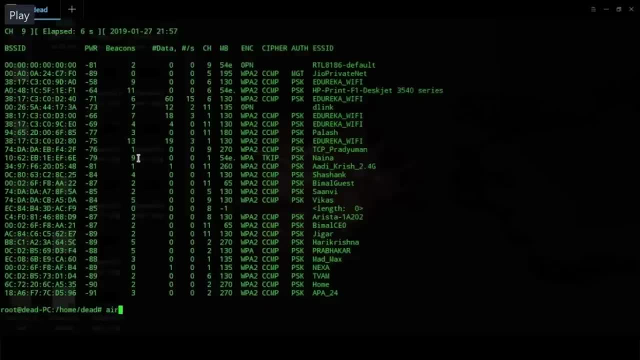 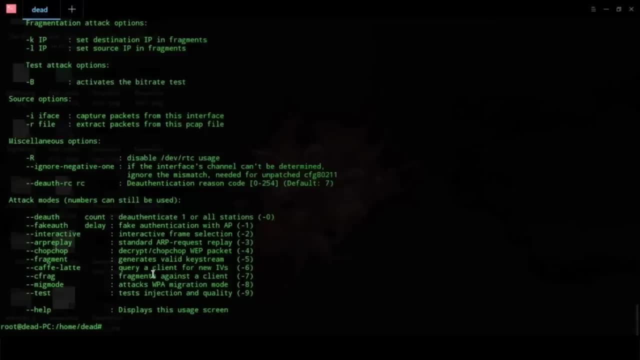 which is a part of the Aircrack NG suite of tools. Now let us just see how we can use Air Replay by opening up the help command. So we go dash, dash, help, and this opens up the help command for us. Now, as you guys can see, 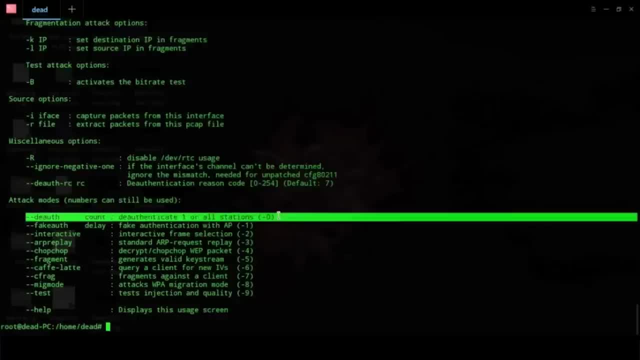 it shows us that we can send a deauthentication message by typing in the hyphen zero, and then we need to type in the count. So what we are going to do is type in hyphen zero, which will send a deauthentication message. 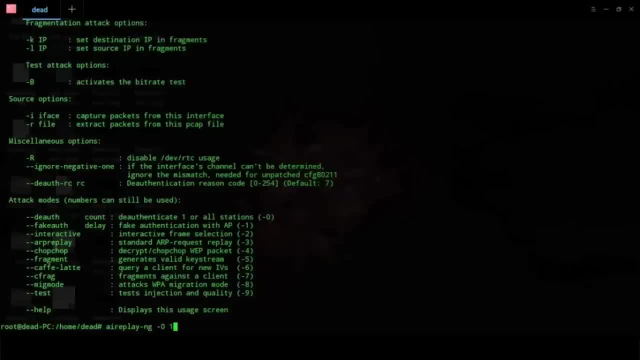 and now we can type one or zero, So one will send only one deauthentication message, while zero will continuously loop it and send a bunch of deauthentication messages. We are going to say zero because we want to be sure that we are deauthenticating everybody. 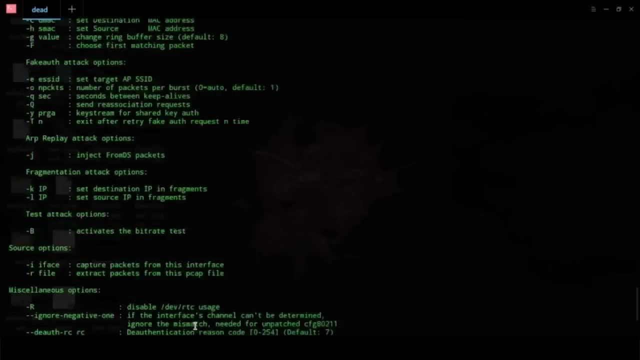 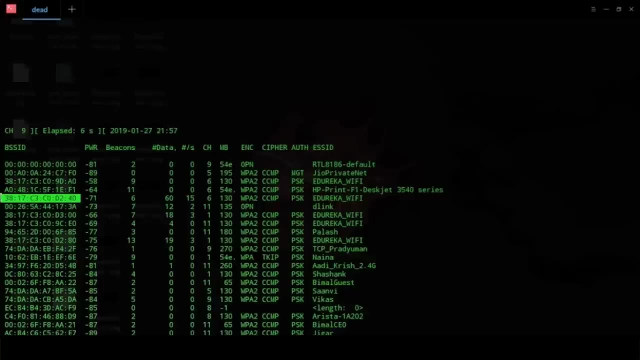 and we can also generally specify the person we also want to specifically deauthenticate, but for this demonstration I'm just going to try and deauthenticate everybody that is there. So what we are going to do is we are going to copy down the MAC address or the BSS ID, as you would know it. 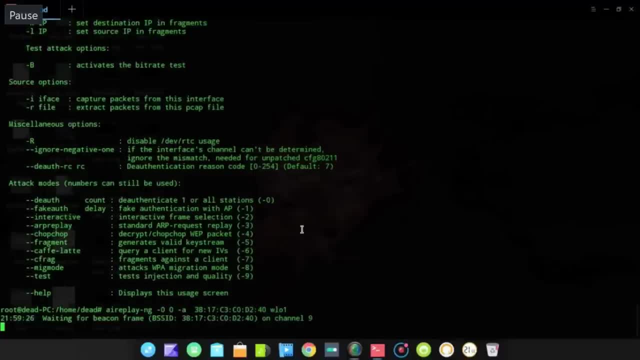 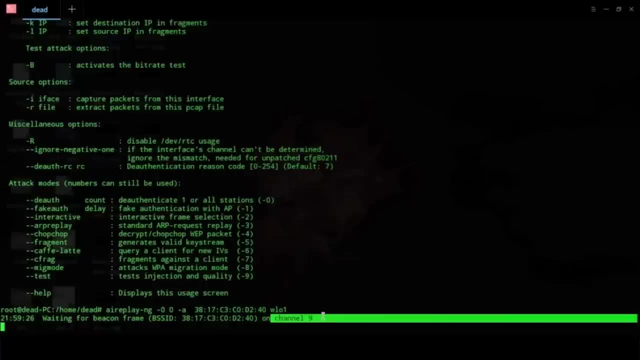 and then we are going to run deauthentication message. Now, as you guys can see, our deauthentication message is beginning to hunt on channel nine. Now, as you guys know, and as I already know, that our BSS ID or MAC address is working on channel six. 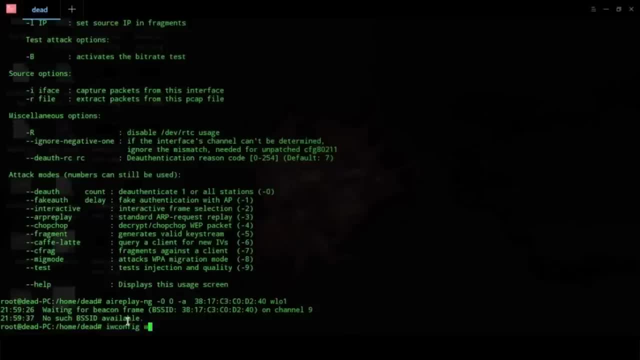 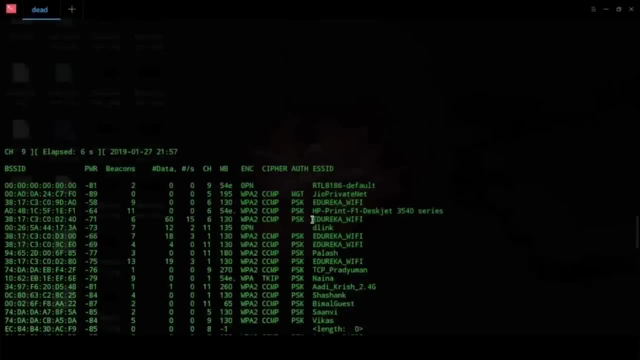 Now we can easily change the channel that our interface is working on by just going iwconfig wl1 and then channel, and then specifying the channel. Now, as you guys can see, our chosen router is working on channel six, so that's exactly what we're going to do. 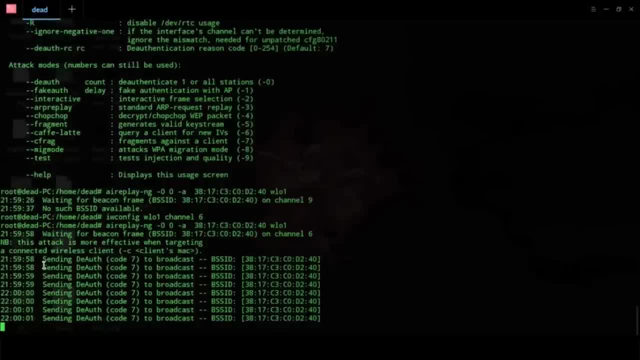 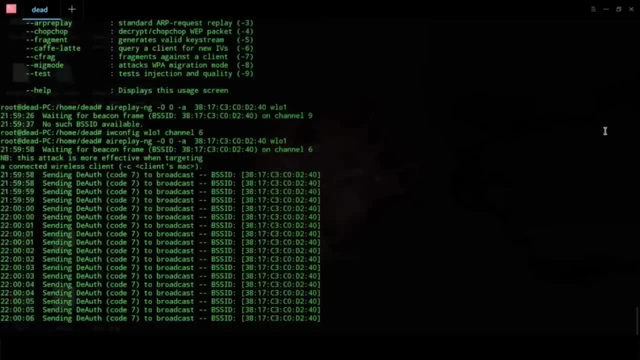 Now, as you guys can see, it immediately starts sending deauthentication codes to the specified router, and this will actually make any device that is connected to that router almost unusable. You might see that you are still connected to the wifi, but try browsing the internet with them. You will never be able to actually reach any site as I'm constantly deauthenticating your service. You will need that four-way handshake all the time and even if it completes, you are suddenly deauthenticated again because I'm running this thing on a loop. 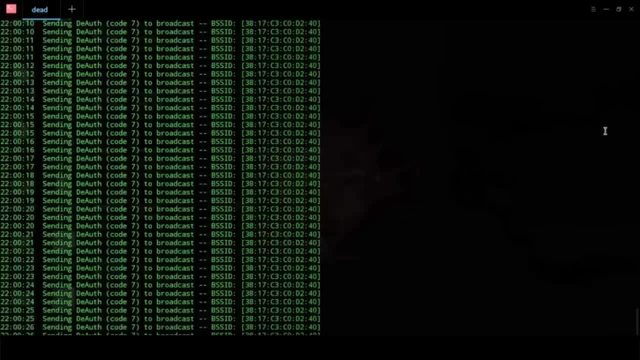 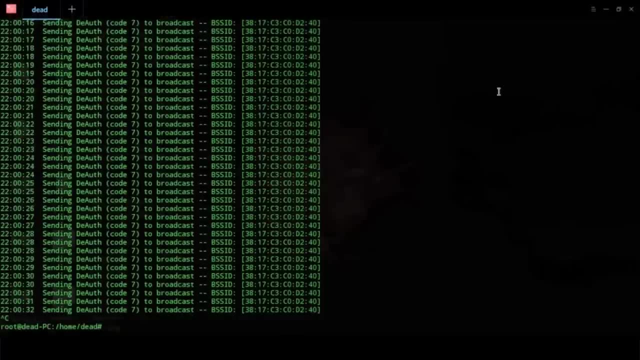 Now you can let this command run for a few moments, or how much of a time you want to DDoS that guy for. Well, this is not exactly a DDoS, because you're doing it from one single machine, but you can also optimize this code. 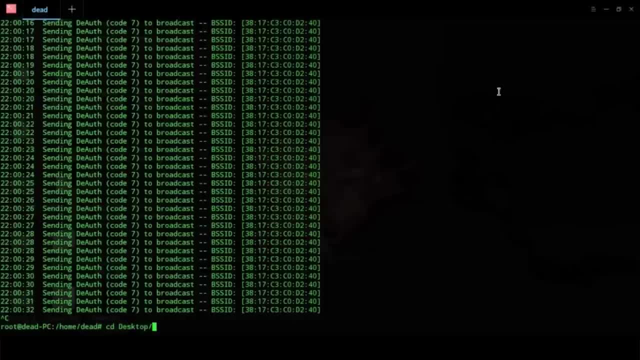 to actually looks like it's running from several different machines. So let me just show you how to do that. We are going to write a script file to actually optimize our code a lot, So this script file will actually automate most of the things that we just did. 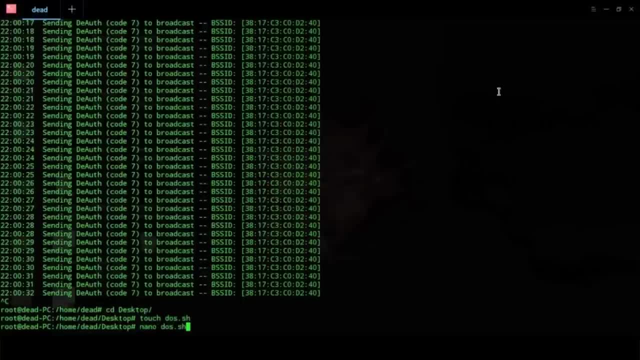 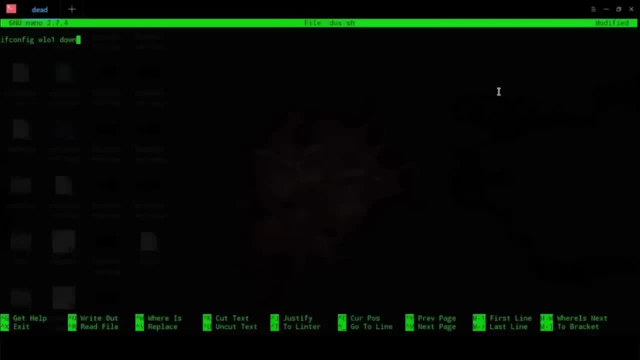 and also optimize a little by changing our MAC address every single time, So we become hard to actually point out. So the first thing that we want to do is we want to put our wireless network card down, and maybe that's not the first thing that I want to do. 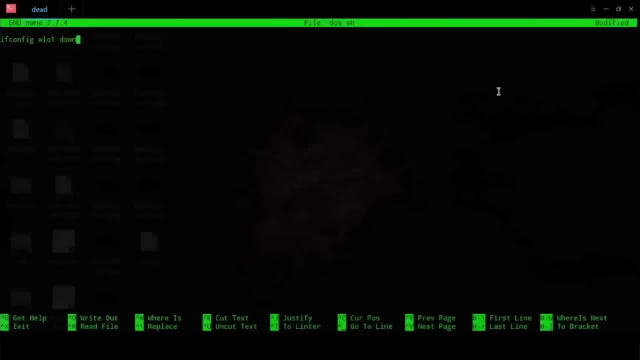 Just give me a moment to think about this. I haven't actually thought this through and I'm doing this on the fly. Okay, so the first thing that we're going to do is we're going to start a while loop that is going to continuously run. 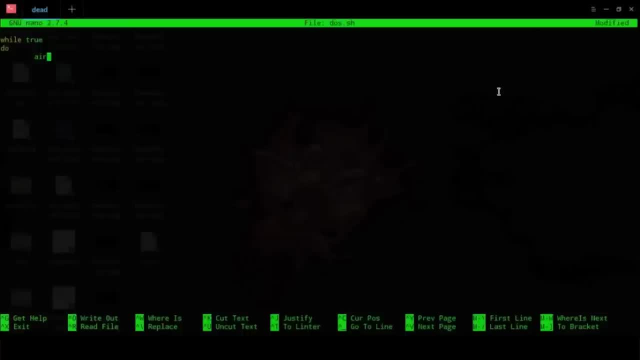 until we actually externally stop it. So we go while true, and then we're going to say do, And the first thing that we want to do is send out a deauthentication message. and we are going to send out a message, we're going to send it around 10 deauthentication messages. 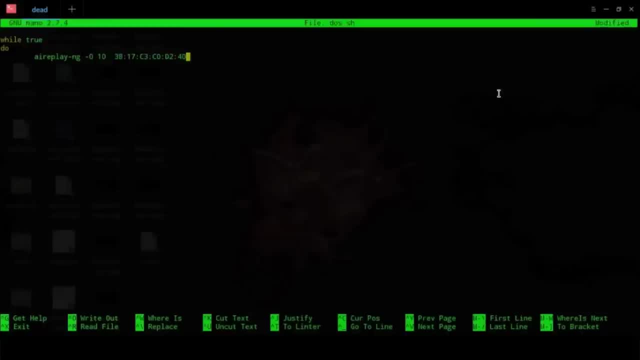 and we want to run it on a specific BSS ID. So that is the BSS ID that I had copied, So let me just put in that and then we just put in the interface that it's supposed to work on Now what we want to do after that. 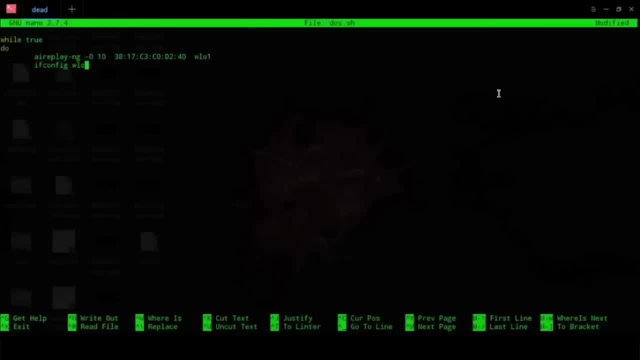 is, we want to change the MAC address after we have sent all these 10 packets. So what we will need to do is put down our wireless network and, as already discussed, we can do that with ifconfig- couple of other one down. 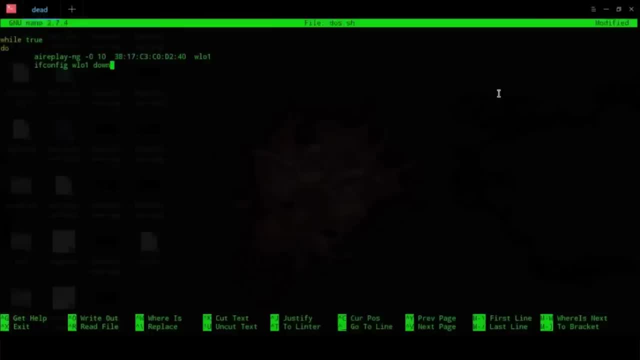 and now what we want to do is change our MAC address. So we can do that with the simple tool that we had installed and saying MAC changer, hyphen R. So let me just open up a quick tab and show you guys how MAC changer actually works. 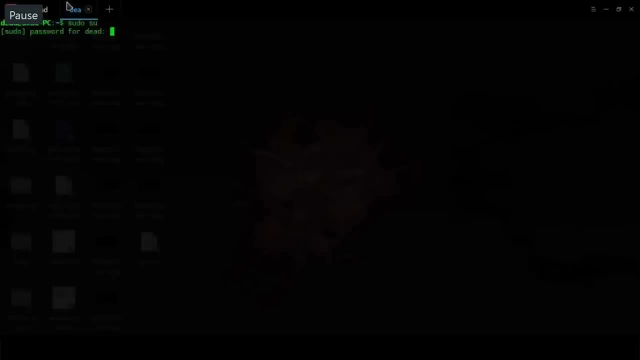 Now you can already check out my other video called the Ethical Hacking Course, which actually covers a lot of topics, and MAC changer is just one of them, And you can check how to use it in depth in that video. But for now let me just give you a brief introduction. 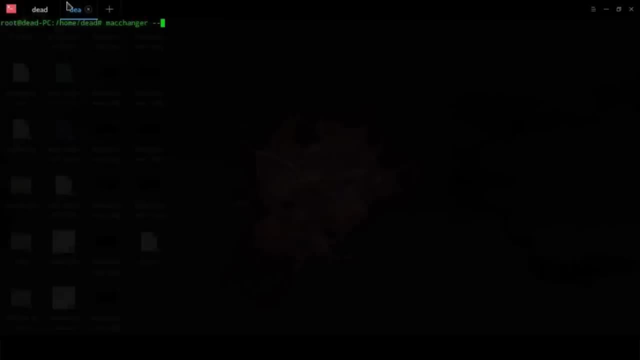 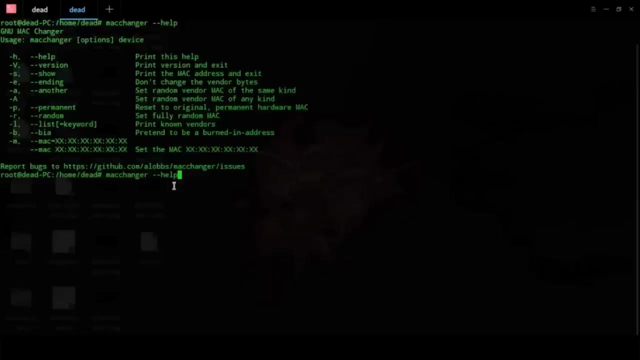 how MAC changer works. The MAC changer will basically give you a new MAC address every time. Let me just open up the help menu for you guys So, as you guys can see, these are the options that are available to us. We can get a random MAC address. 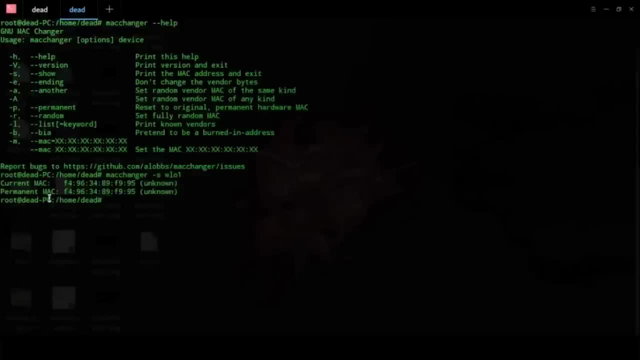 We can also tell it to show our MAC address, and we also have to specify the interface when we want to show us the MAC address. Now let me just generate a new MAC address. So you see out here that interface up or insufficient permissions is being shown. 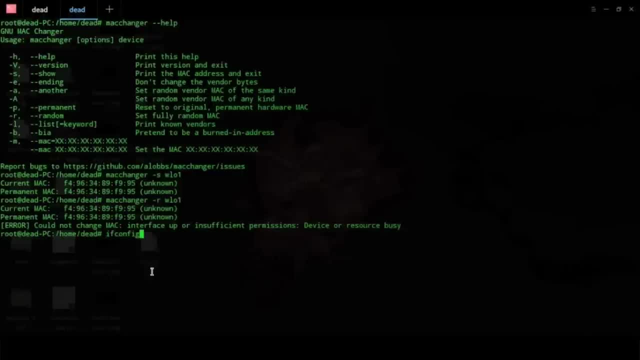 So this means we always have to put down our interface first. So let me just do that quickly. I've gone, pick WL01 down, and now what we want to do is give ourselves a new MAC address and- boom roasted, We already have a new MAC address. 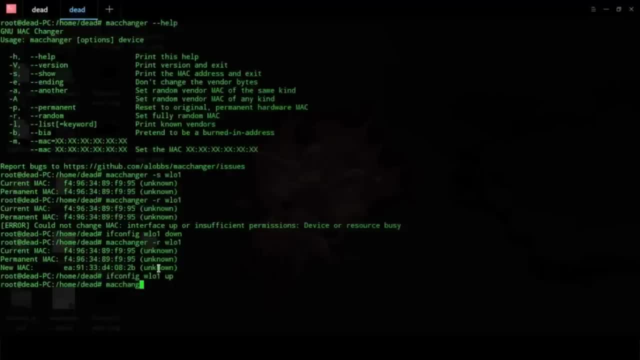 as you guys can see from the new MAC part. Now, if we put back our network interface card and then try and show our MAC address again, we see that our current MAC and our permanent MAC are two completely different MAC addresses, And our current MAC and the new MAC are identical. 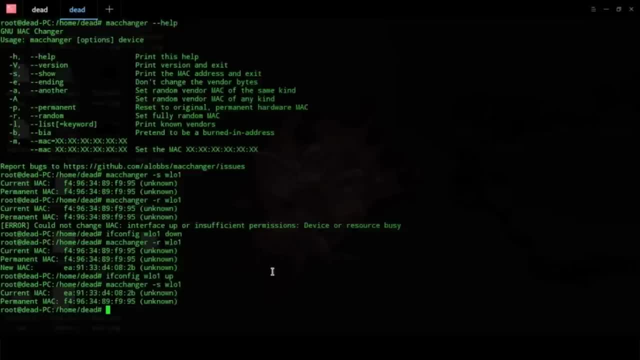 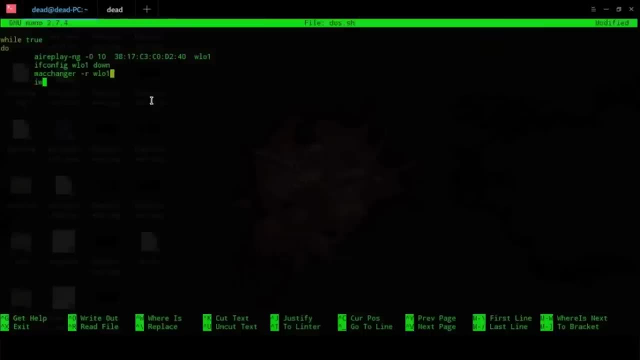 So this is how you can actually generate new MAC addresses to spoof your own identity on the while, And that is very useful in this case, because the person you're attacking will be so confused as to what to do because your MAC address is changing every time. 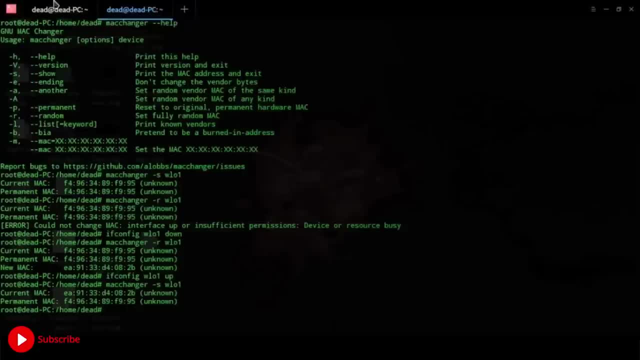 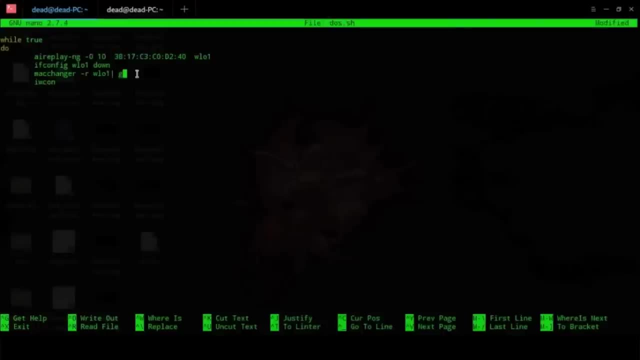 And there's no real solution to the situation that you're creating for them. At least, I don't know of any solution. If you do know how to stop this for yourself, please leave it down in the comment section below and help the world a little bit. 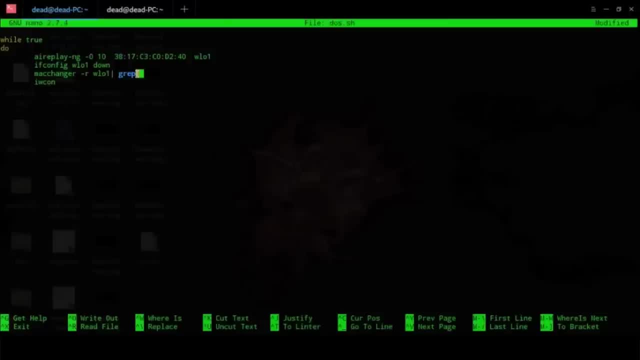 Now we want to also get to know what our MAC address is every time. So let me just pipe my function through the whole thing and let me just try and grab the new MAC address. So MAC changer are WL1 and grep MAC. And then we want to put our info card in the monitor mode. 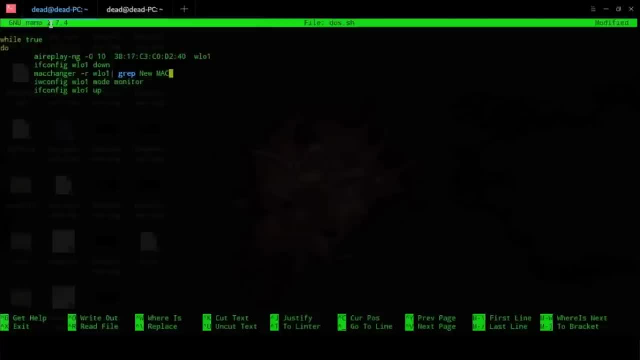 And then we also want to put up our network interface card. Now, what we want to do out here is optimize it So we can't be attacking constantly. So let us put a sleep timer, So this will make our program sleep for a particular amount of time. 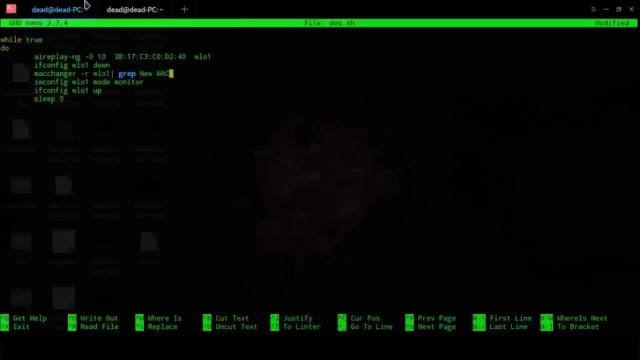 I'm going to make it sleep for five seconds. So after every five seconds it's going to send that particular BSS ID, Then it's going to send that particular BSS ID, Then the authentication messages, Then it's going to bring down my interface card. 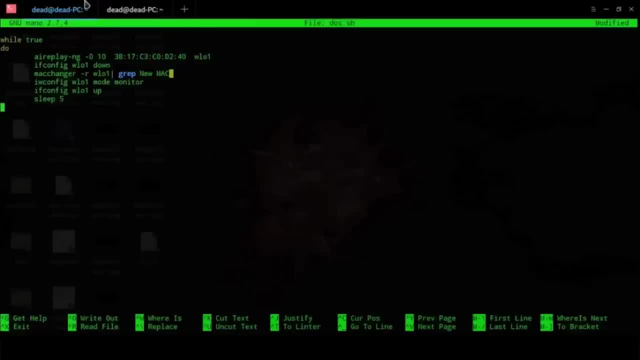 It's going to change my MAC address. It's going to put back the interface card into monitor mode and sleep for five seconds and then repeat the entire process, And to end the script let's just say done, So that will denote when the loop is done. 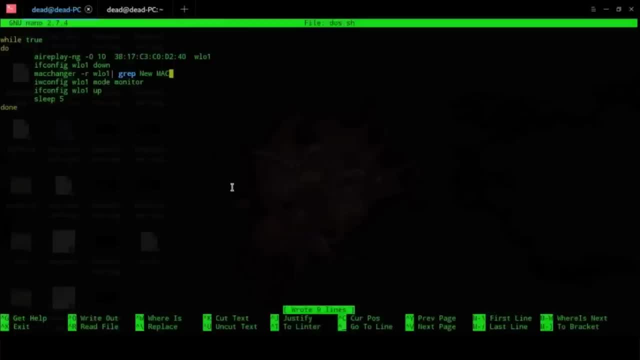 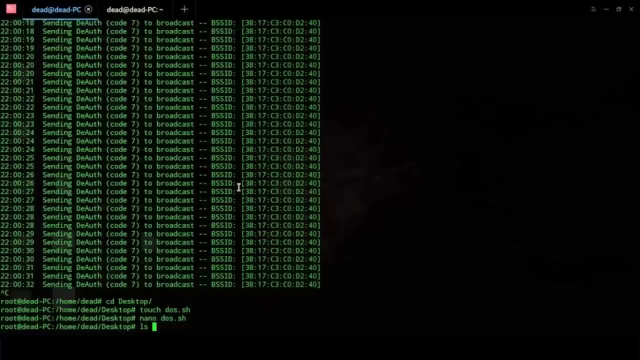 Now let me just save it. Control O, control X to exit. And there we go. Okay, so, first of all, to actually run this need to give it sound, I'm going to give it some more permissions. So, as you guys can see, we already have it. 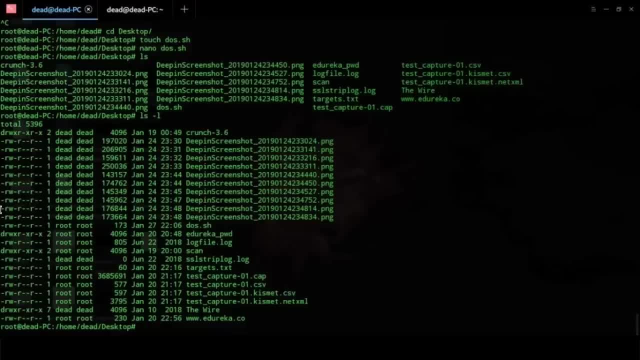 Let me just put it in a much more readable format. Okay, so, as you guys can see, our DOS, DOS SH doesn't really have executability, So we can do that with command CH MOD. So I'm going to give it some executable permissions. 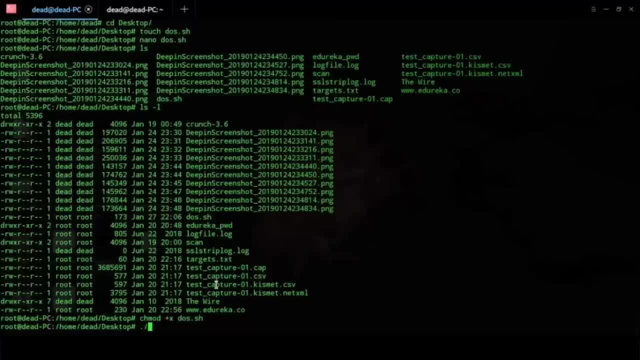 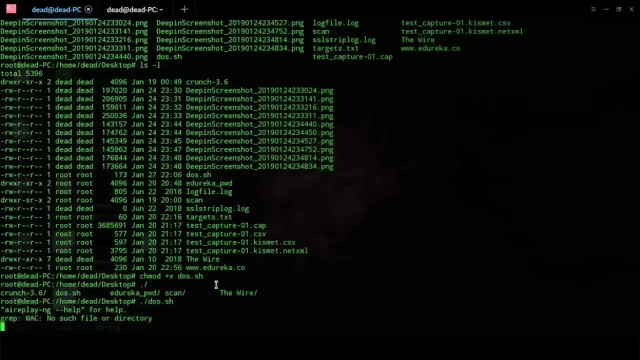 So CH MOD plus X and then the name of the file. So this will actually change our DOS, DOS SH, into a executable bash script. Okay, so it seems that we have done some error, So let's just go back into our bash. Let's go back into our bash script. 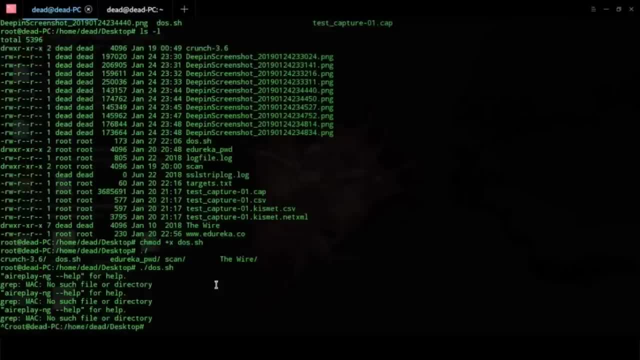 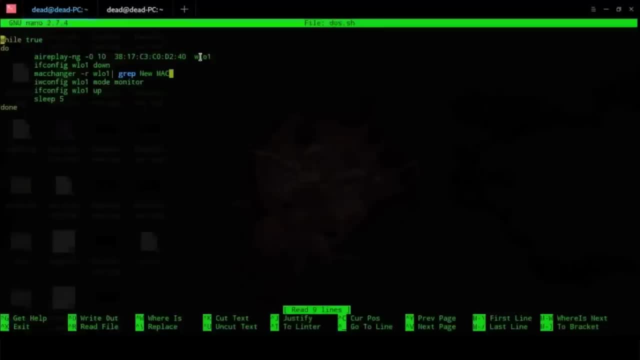 and check for the error that we have probably done. So nano, DOS, DOS SH, DOS dot SH. Okay, so the thing that I am missing is that I forgot the hyphen A that I'm supposed to put before putting the BSS ID in the air replay ng. 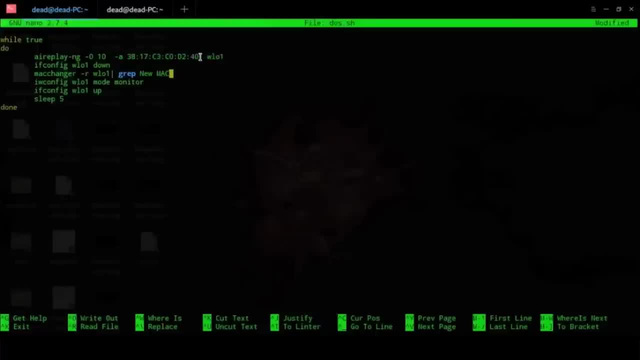 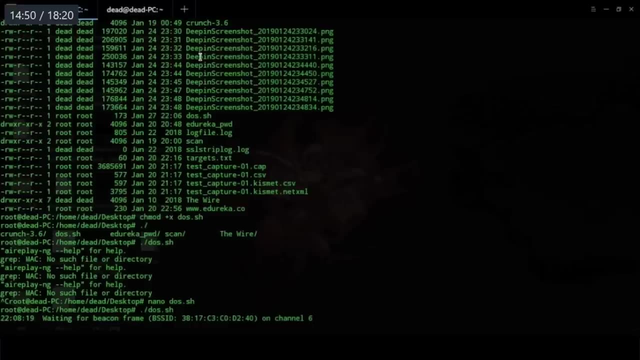 part of the code, So let me just go ahead and quickly do that. Okay, so now that that is done, let me just save it and quickly exit and see if this thing is working. Okay, so now we are trying to work out our script. 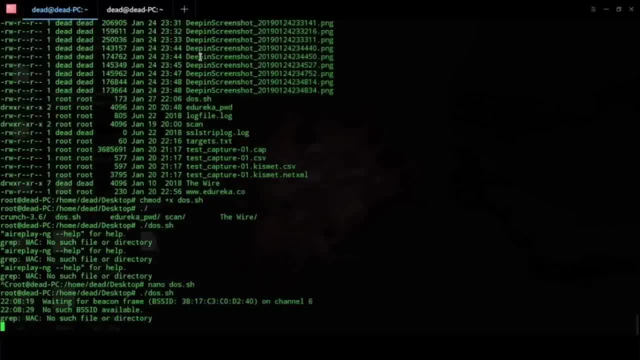 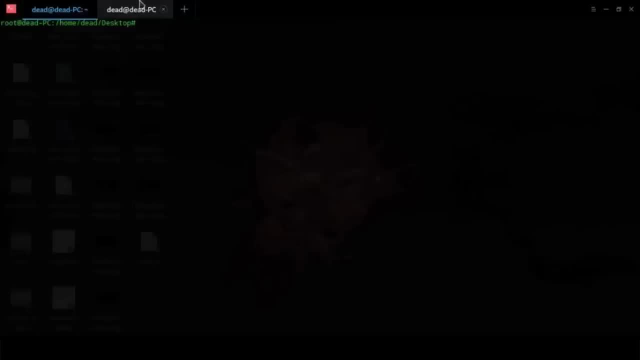 Now you guys should know that this edureka wifi is my company's wifi and I have complete permission to go ahead and do this to them. Also, my company's wifi is kind of secure, So every time it senses that, a deauthentication message. 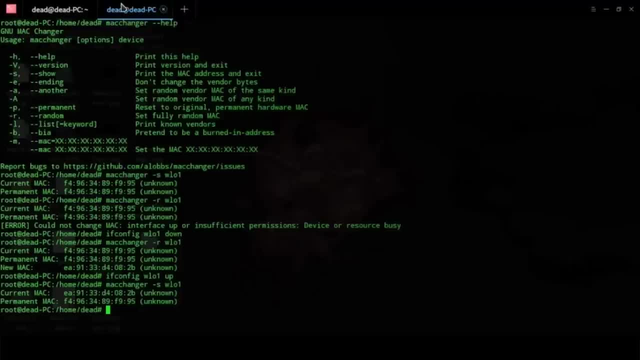 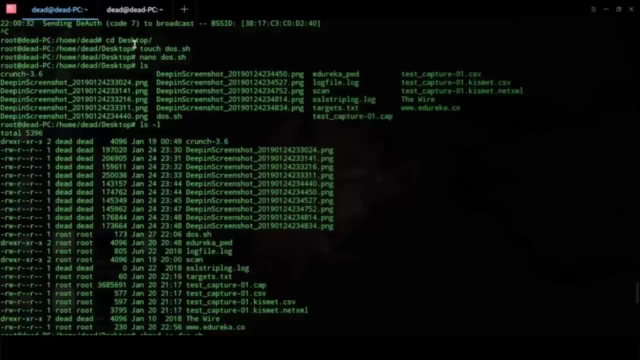 is being sent like that, it kind of changes the channel that it is working on. So these guys are really smart- smarter than me most of the time- And this time I'm just going to try and force them to work on channel. 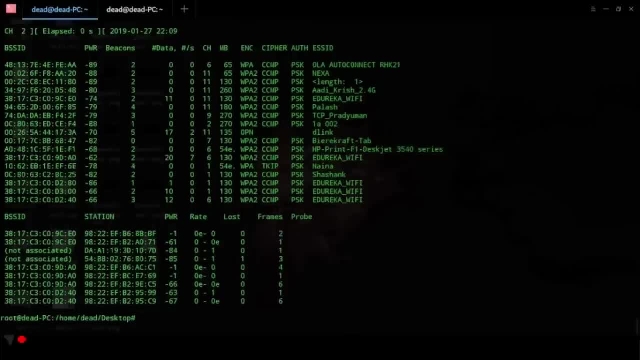 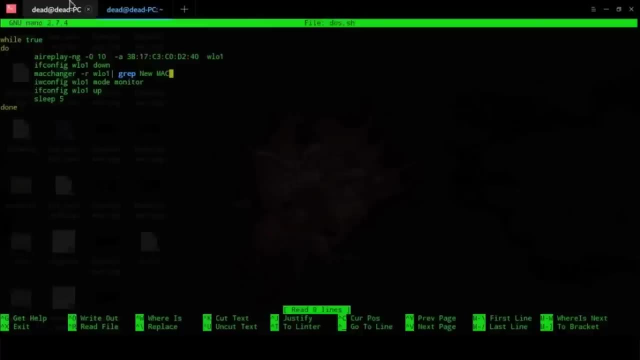 So let me just go ahead and run my script once. Okay, so let me just check that they're still working on channel six. Yep, they're still working on channel six. Let me just check my script once, if it's correctly done. 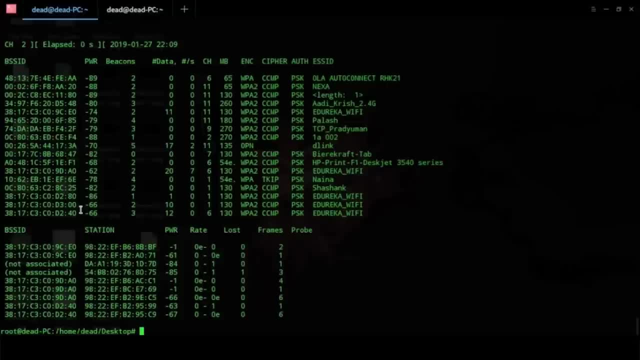 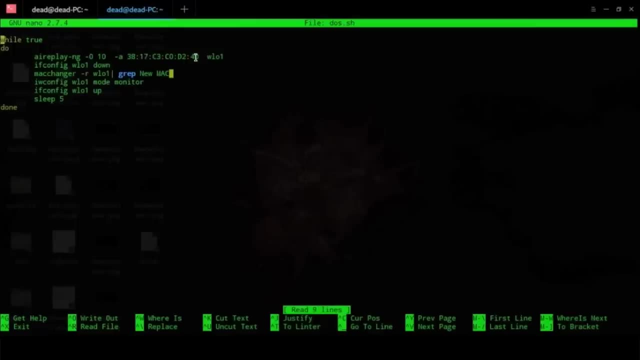 If I have the perfect Mac ID, let me just copy in the Mac ID, just to be sure once again. So there you go, we've copied it. Let's go into the script and let's paste it out. Okay, so now that that is done and we have Mac IDs, 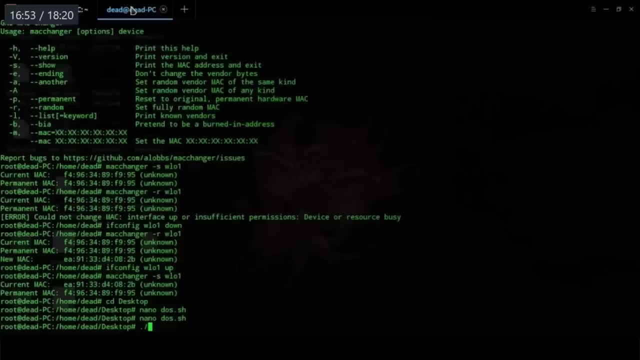 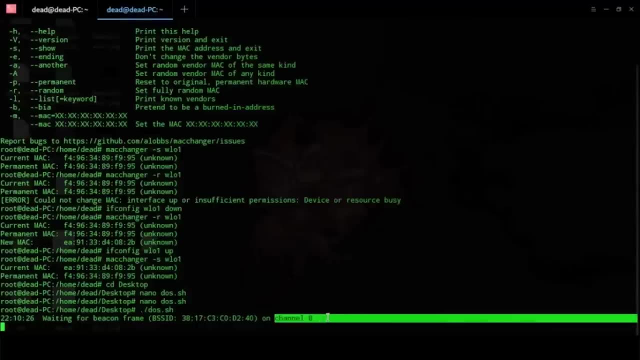 and everything set up properly. let me just show you how to run the script. So you go dot and backward slash and then you said dot, dot, sh. Now you see that our thing is working on channel eight. So this will definitely not work and it'll say that BSS ID is not there. 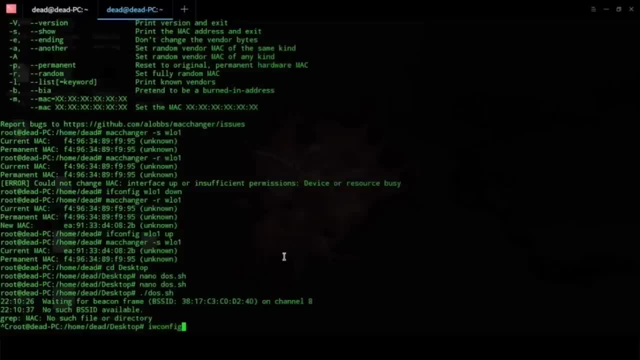 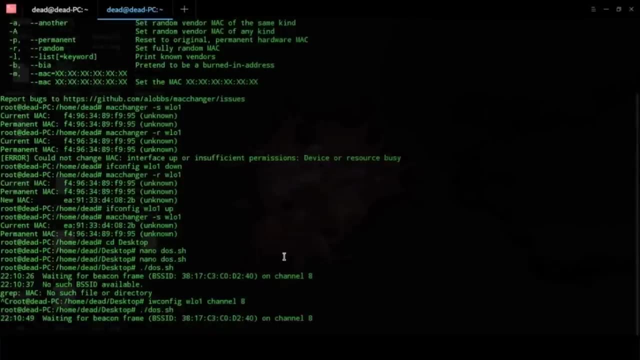 So what we need to do, as I had showed to you guys earlier, we can go iwconfig wl1 and change the channel to channel six. Oops, I changed it to channel eight again. This will not work. I'm sorry, that was my bad. 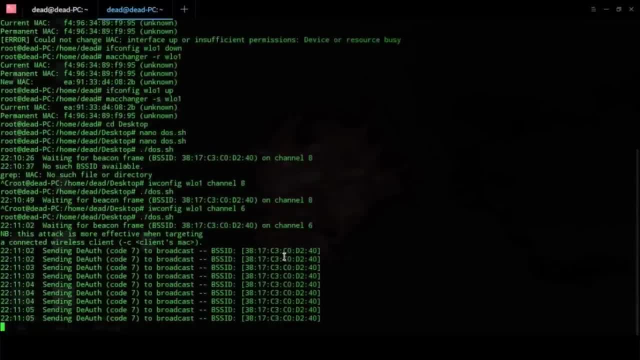 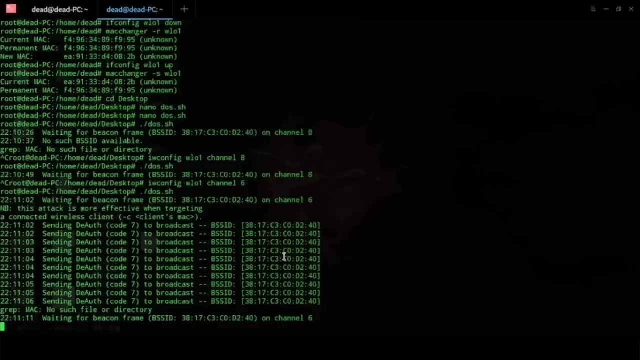 So now that we have changed it to channel six, you can see that it is sending everything immediately. Okay, so that is actually running our script very well And, as you guys can see, the security measures that are taken by my company, it will not always work on channel six. 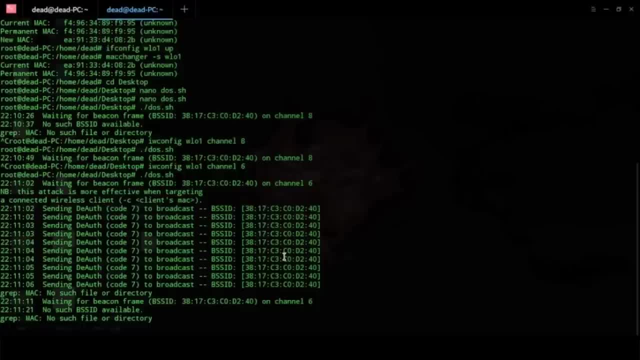 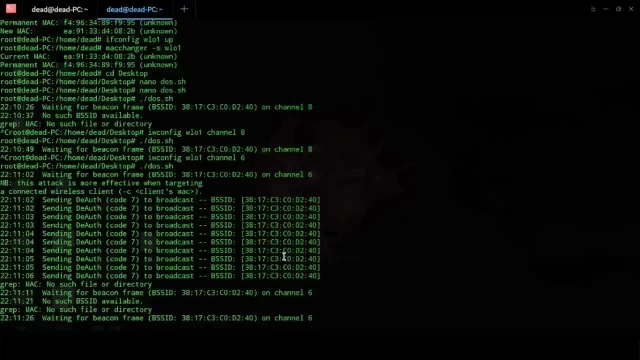 It'll keep rotating now until it finds a safe channel. So it really can't find a safe channel, I will always be dosing on channel six and it will run sometimes and it won't run sometimes, but mostly with unsecured wifi that is running. 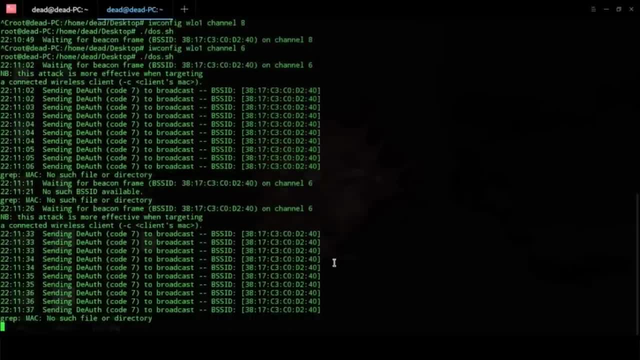 at your home. mostly this will work 100% times. So let me just stop this, because my company will go mad on me if I just keep on dosing them. So this brings us to the end of our demonstration. This is how you can always dos your neighbors. 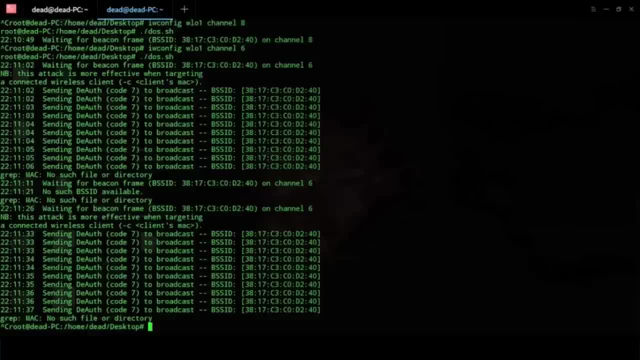 if they're annoying you, but remember, if you're caught, you could be prosecuted. So this was about how DDoS works, what DDoS actually is and the different types, and how you can do one on your own with your own system. 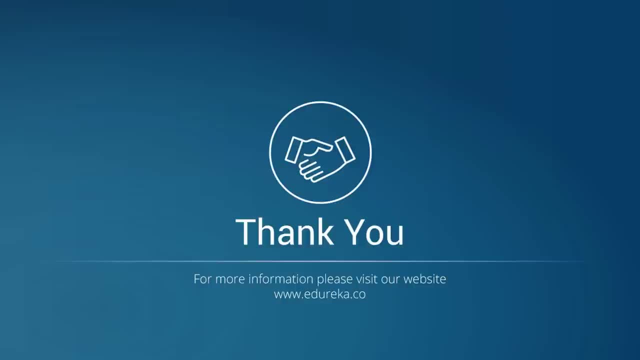 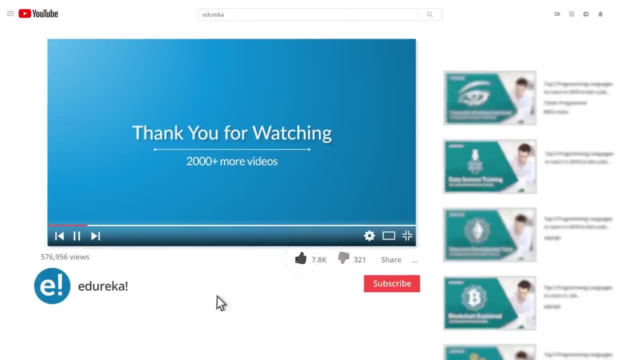 Okay, so that's it for me for today. I'll meet you guys in the next tutorial video. Goodbye. I hope you have enjoyed listening to this video. Please be kind enough to like it and you can comment any of your doubts and queries. 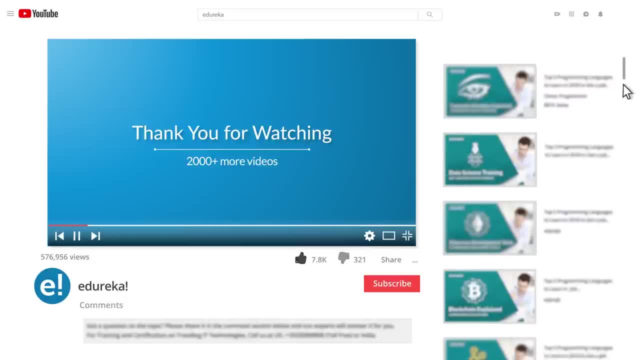 and we will reply them at the earliest. Do look out for more videos in our playlist and subscribe to Edureka channel to learn more. Happy learning.